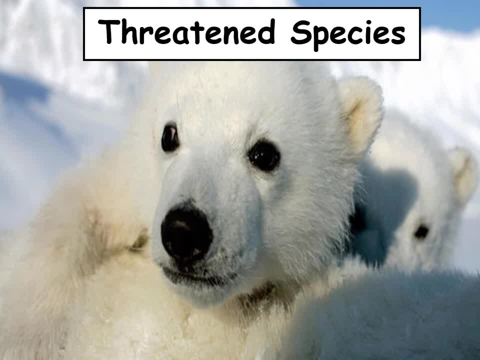 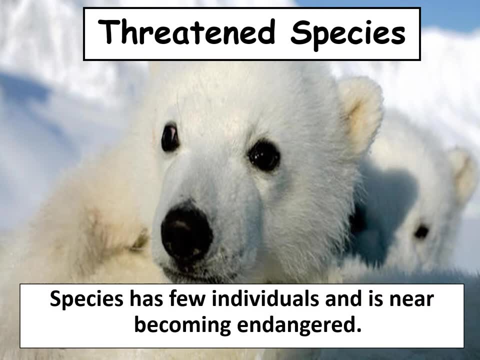 Endangered Species Act. there are some terms that you should probably be aware of. So a species can be listed as threatened, and if the species is threatened, that means it has very few individuals and it is almost endangered. So the population is in trouble, but not huge trouble Like we're. 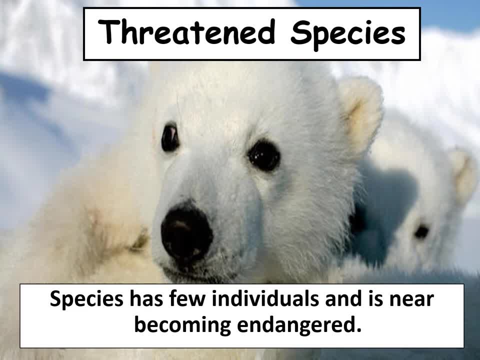 noticing there are decreases with the population and it could be an issue. So a good example of a threatened species here in the United States is the US Endangered Species Act. It's a very common term that is used in the United States is the polar bear. Another example of a threatened 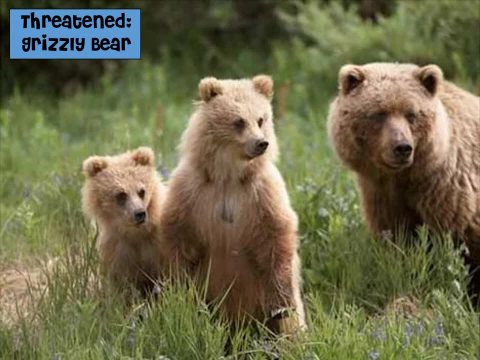 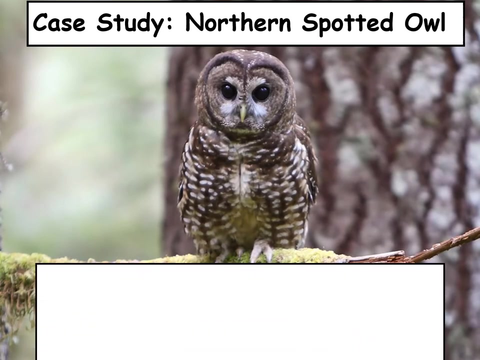 species is the grizzly bear. It is listed as threatened on the US Endangered Species Act And, remember, these are species that need to be or reside in the United States. The northern spotted owl is also listed as threatened on the US Endangered Species Act And this is primarily. 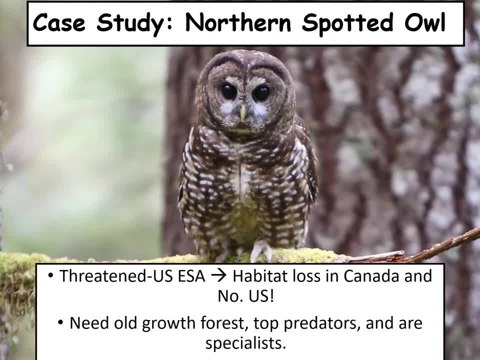 due to habitat loss in its forests. The problem is that this owl needs a lot of old growth forests and those really are only found in the Pacific Northwest. They are the top predators of the area and are specialists, So they do have a specialized diet and so forth. So all of these three things. 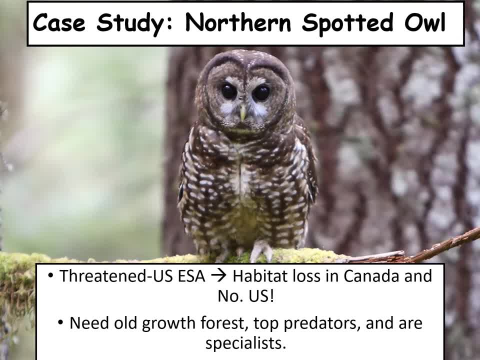 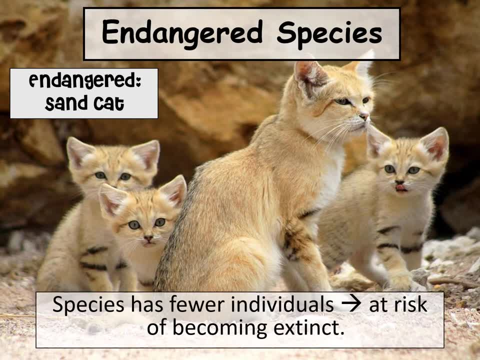 really have contributed to its threatened status. Endangered species is one in which the population is in real trouble. There are not very many individuals left of that population and it is at risk of becoming extinct. So an example of an endangered species here in the United States is the sand cat. Also another example is the white. 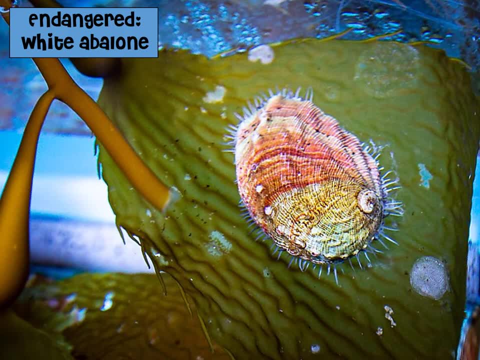 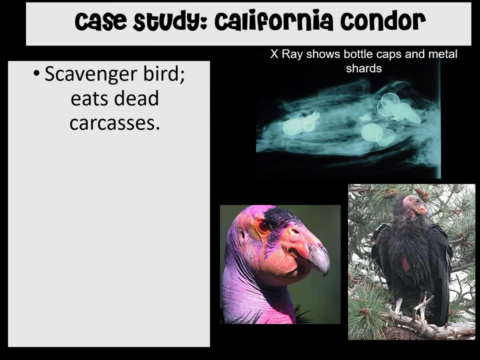 abalone. We have these here off the coast of California, And the California condor is probably the most notorious endangered species. It is a scavenger bird and it does eat dead carcasses. In 2005,, there were only 273 individuals of the condor left. This led scientists to pull them. 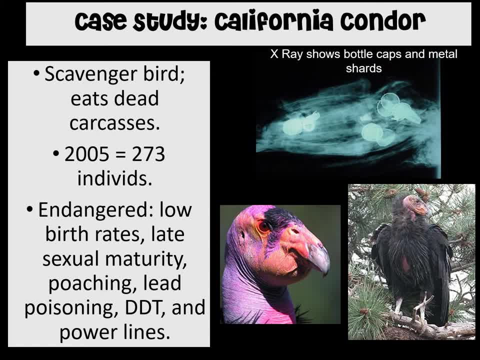 out of their natural habitat because it was just too dangerous for them to be in it. They rehabilitated them, They bred them in captive breeding programs And they are still currently listed as endangered. but they're doing much better. So it doesn't help that they have very low birth rates and late sexual maturity, So that does not. 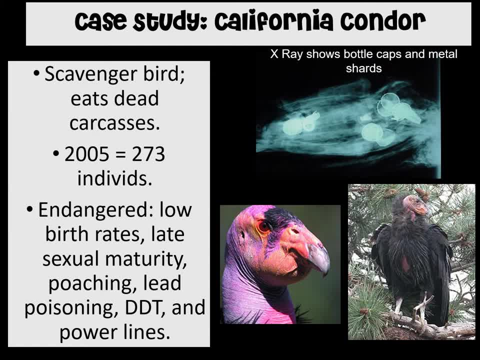 increase their populations very quickly. What was causing the deaths of these condors was a variety of things: Poaching for their feathers, lead poisoning from bullets from hunters, DDT from pesticide usage and, unfortunately, sometimes they would just fly into power lines. Sometimes, when 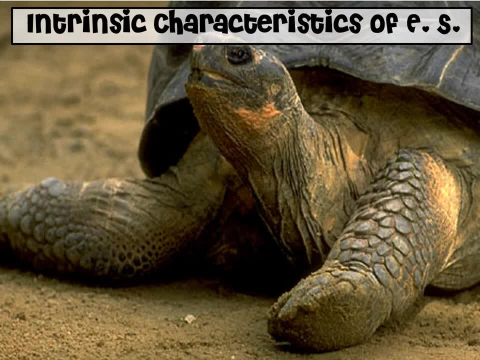 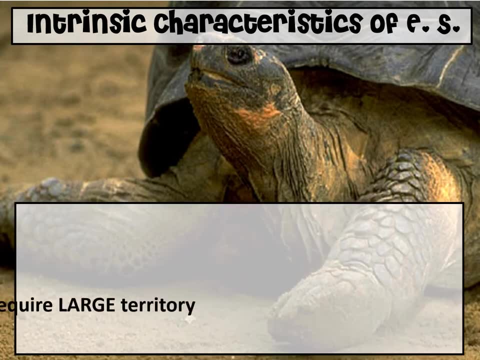 you want to rehabilitate endangered species, they would just fly into power lines, And they would just fly into power lines. So there are things that reside inside of them, intrinsic characteristics that make it very difficult to bring the population back. So, for example, some of these species you're 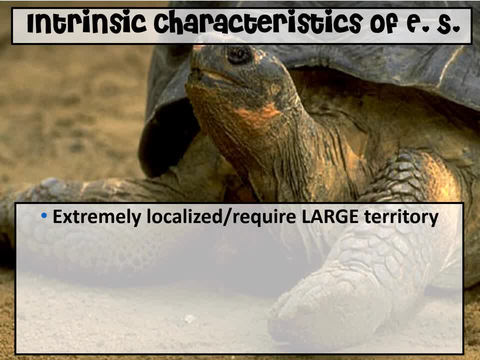 going to notice, are extremely localized. They're only found in one place, or can be endemic or require a large amount of territory. They may have low birth rates, So instead of producing maybe 50 babies at one time, they'll only do one or two. They sometimes reside on islands or are just very 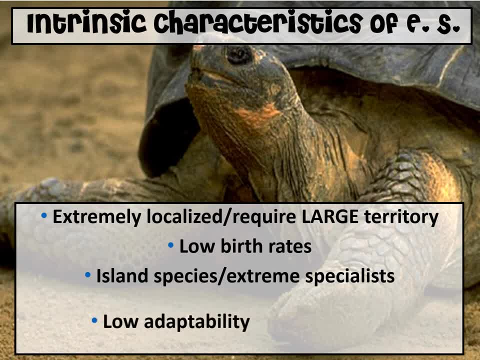 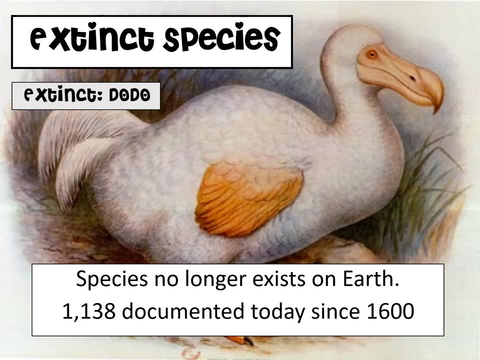 extreme specialists, So they require a very specialized diet. They don't adapt well to changing conditions And sometimes it takes them a very long time to reach that sexual maturity. Another category used is the extinct species category And I think you all probably know that. 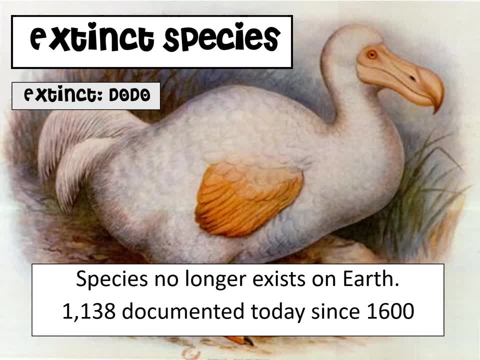 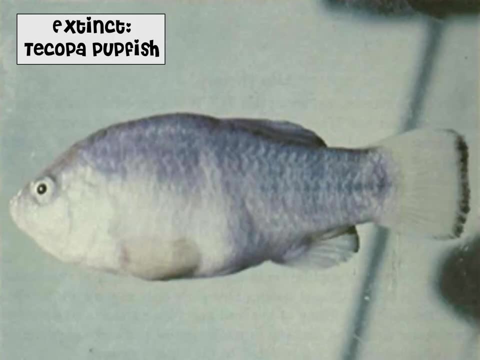 this is when the species no longer exists on Earth. There have been about a thousand documented, But of course we all know that many more have passed on without us knowing, And so a very famous one is the dodo species. Here are some examples of some extinct. 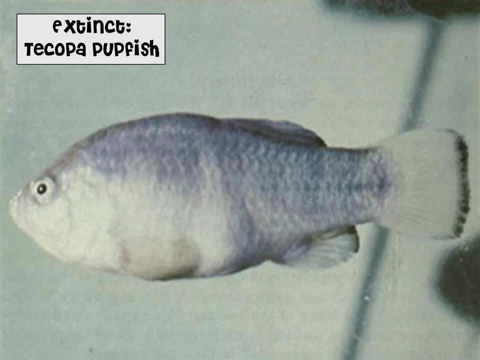 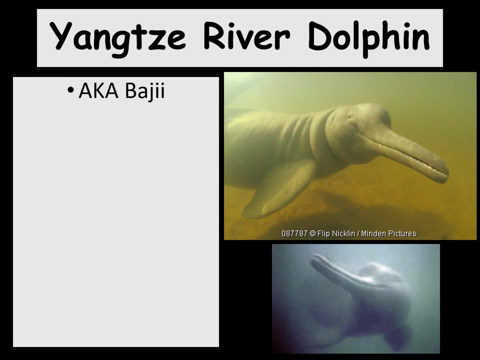 species. So we have the Tacopa puttfish, which is a very small fish, And the Yangtze River dolphin has been officially declared as a extinct species- I hope I'm pronouncing this right- sometimes known as the Baji, And the last sighting of it was in 2004.. You might be asking what caused. 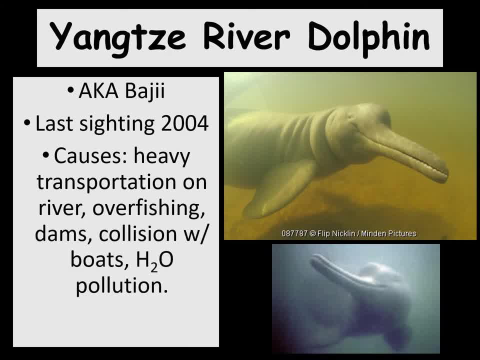 its decline. Well, it lived in the Yangtze River And there was heavy transportation on this river, lots of big boats and collisions. We have overfishing in the river, Dams are being built, like the Three Gorges Dam is on this river- and water pollution. So all of these contributed to. 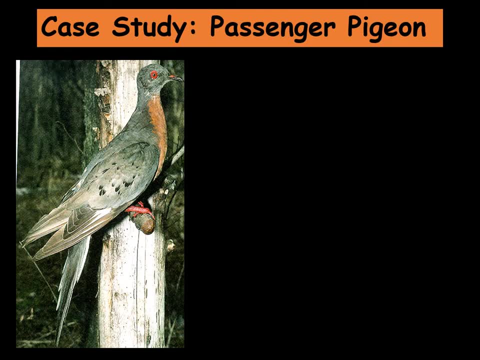 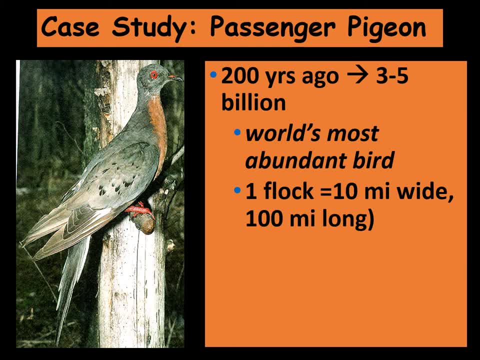 very, very, very powerful bird. It's the passenger pigeon, And there were approximately three to five billion passenger pigeons on this earth about 200 years ago And we killed them all, Mainly sometimes sport hunting, maybe eating. This was the last one. It is currently stuffed on. 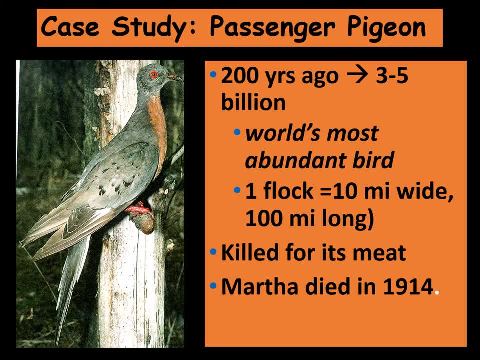 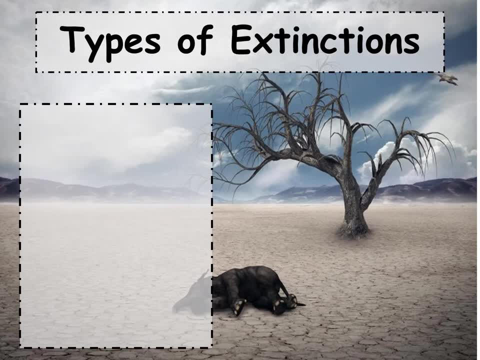 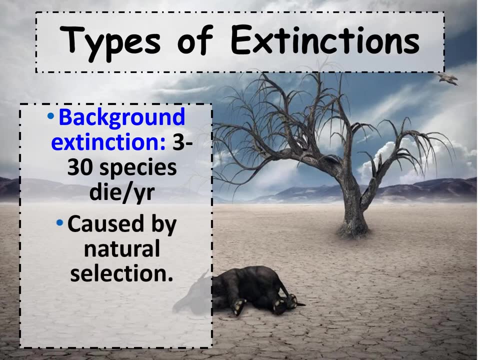 display, But Martha was the last one ever in the United States and it died in 1914.. different types of extinction. So let's compare the two. The first one is a background extinction, and this is where about three to thirty species die each year, and it's thought that these species 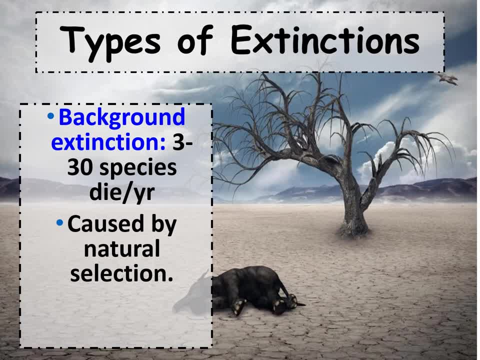 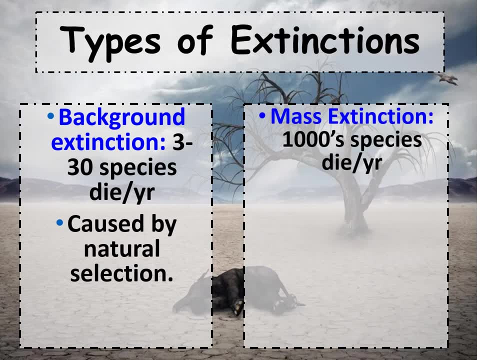 die out due to natural selection. So nature is selecting which organisms are best fit for their environment. Compare that to a mass extinction. A mass extinction is where you have about a thousand species dying each year, and it's usually caused by some sort of environmental change We've had. 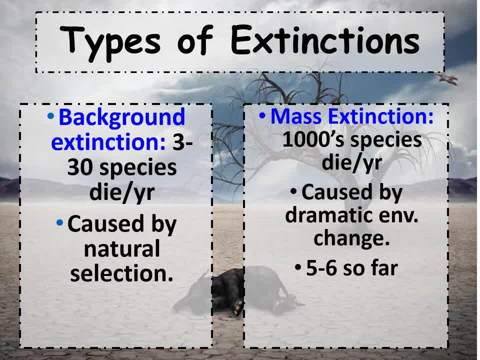 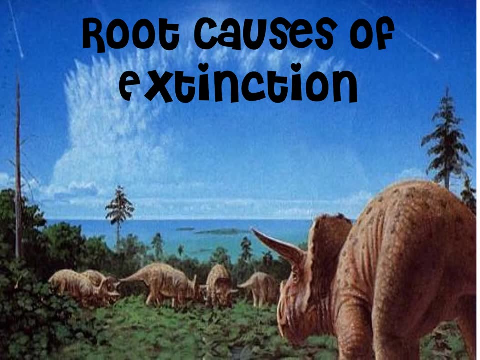 about five to six so far. One example would be like the wipeout of the dinosaurs thanks to the meteor, and some scientists will argue that humans are causing the sixth mass extinction here on earth. So really, what is causing pretty much all the extinction here on earth? We got too many people. 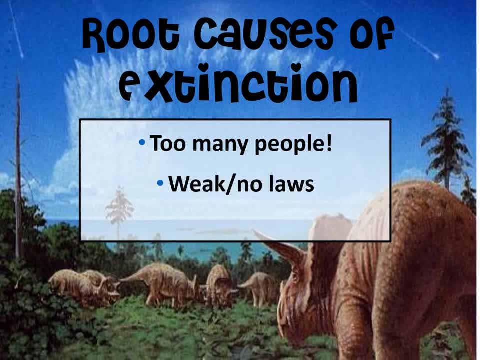 on this earth: not enough natural resources, we have laws that don't really support species and, lastly, we have very high consumption resources. We have laws that don't really support species and, lastly, we have very high consumption resources. We have laws that don't really support species and, lastly, we have very high consumption. 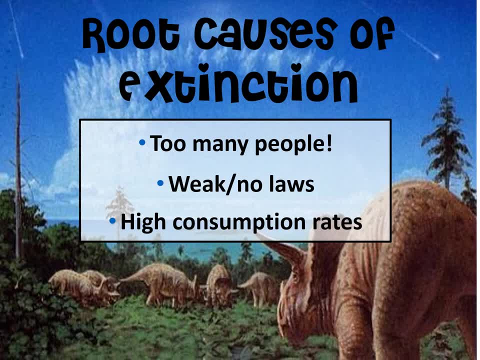 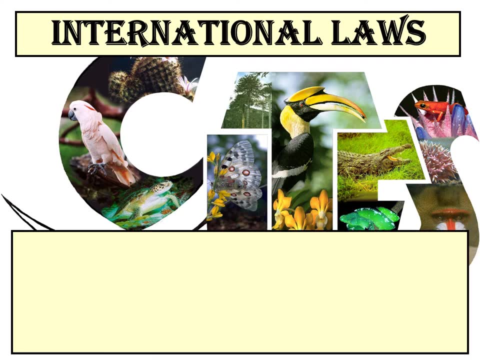 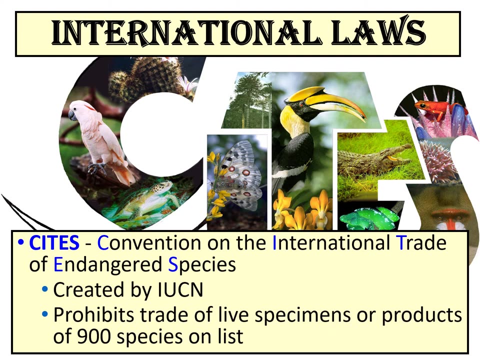 rates. We tend to consume things we don't necessarily need. There are some international laws that exist to protect species. An international law that you should probably know about is CITES. It's the Convention on the International Trade of Endangered Species and what this list does. so if the organism is put on this list, it does prohibit the trade of these. 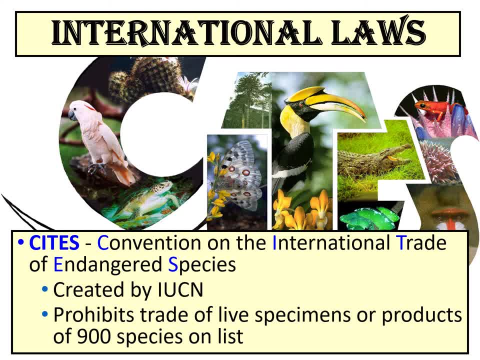 life specimens or products to any country. that, of course, abides by CITES. So if you're looking at the CITES list, it's not going to prohibit the trade of these life specimens or products to any country. that, of course, abides by CITES. 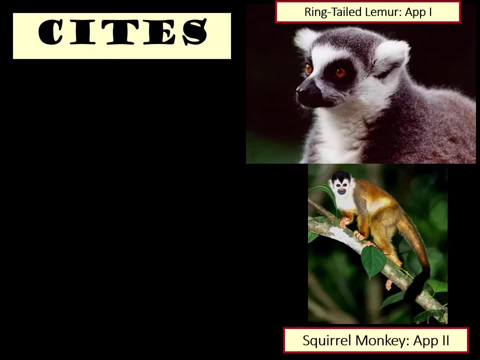 So, if you're looking at the CITES list, it's not going to prohibit the trade of these life specimens or products to any country that, of course, abides by CITES. Now, instead of using threatened, endangered and extinct, like the US Endangered Species list uses. 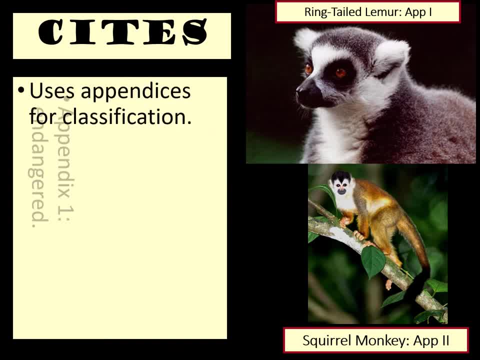 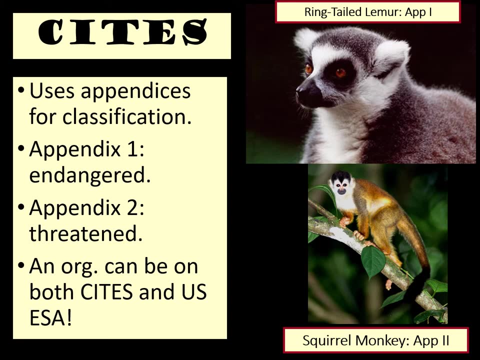 it uses what are called appendices, And so, for example, appendix one means endangered, and if you're appendix two, that means you are threatened, And so an organism can actually be on both lists. So it can be on the CITES list, so international trade, and it can be on the US Endangered Species list. 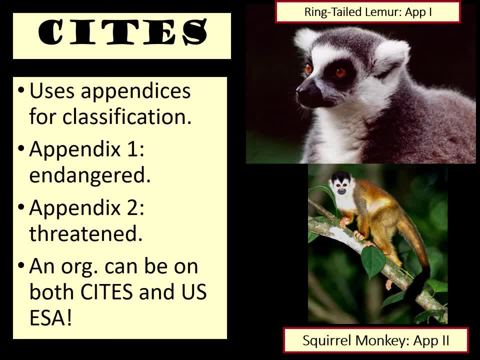 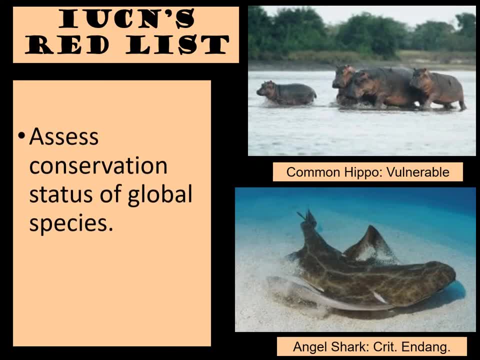 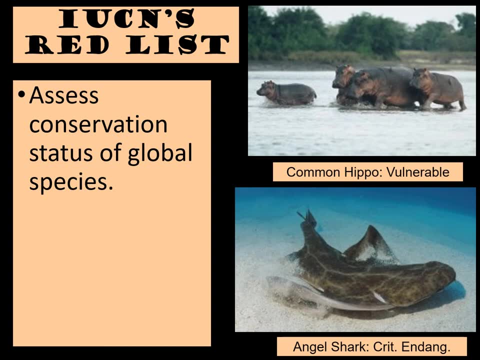 And then, of course, it can be on the United States Endangered Species list if it resides in the United States. There's also the IUCN's RED list, and the RED list uses its own terminology. This RED list was created to assess the conservation status of different species. 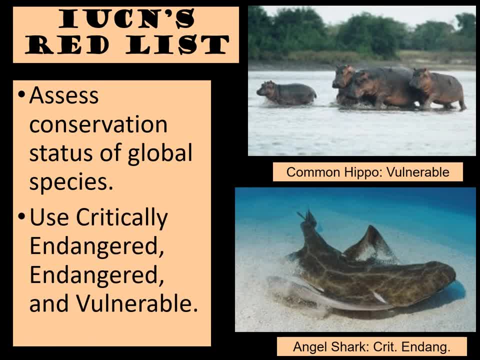 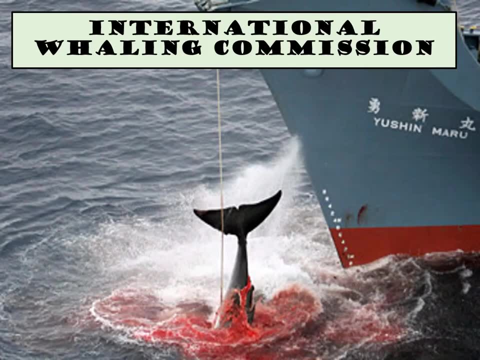 found around the world and they used the words critically endangered, endangered and vulnerable. So if you want to think about it like vulnerability is thickened, Endangered is endangered And critically endangered is an endangered subspecies. critically endangered means: ooh, that organism is in trouble. The International Whaling Commission. 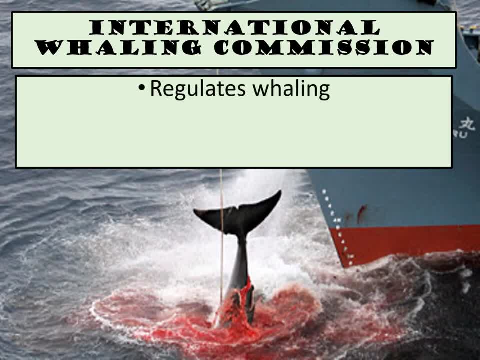 was also created to regulate whaling that was taking place around the world, And so it does ban, of course, whaling and gill netting and purse sayings that are used, And then keep in mind, though, that not all countries have signed on to this whaling commission: Japan, Finland, 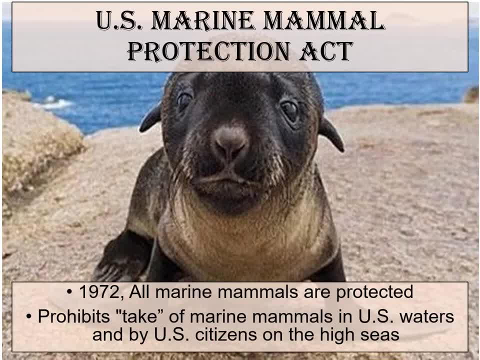 and Iceland have not signed. And lastly, let's not forget about the United States Marine Mammal Protection Act. This was established in 1972 to protect all marine mammals in the United States waters. So all of them are protected. And what does that mean? You cannot take any marine mammals. 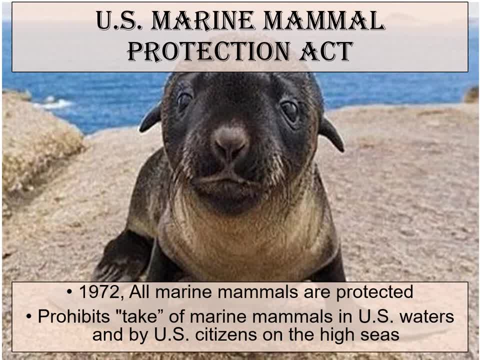 you cannot harm them or hurt them in any way. They are definitely protected by law. Okay, everyone. that concludes our little talk on endangered species. I hope that was great Talk to you later.